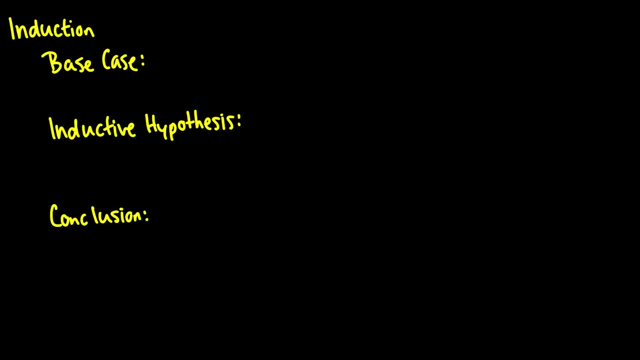 pretty much everywhere to prove that something holds forever- And that's the most important part- is for something to hold forever. So what is induction? Well, induction has three main steps. It has a base case, which this is basically that the first thing is true, And I will compare this. 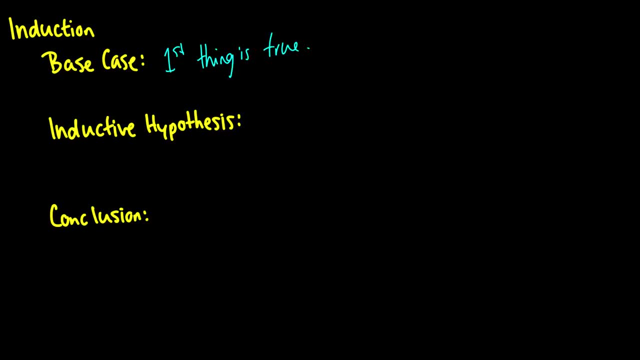 to going up a ladder. So suppose you have the beginning of a ladder and you want to make sure that there is a first step on the ladder. So this first step going up is the base case. Now the interesting thing about the induction: 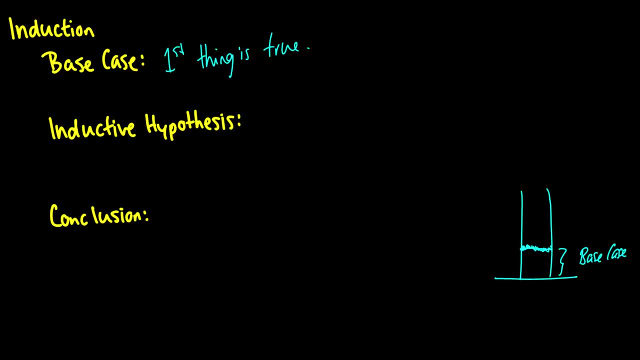 which is the second part, is that you assume something is true for any number less than or equal to some number- k. So what we're doing here is we're going somewhere up the ladder and we're picking some arbitrary step, And this is k, And then you want to show that k plus 1 is true. 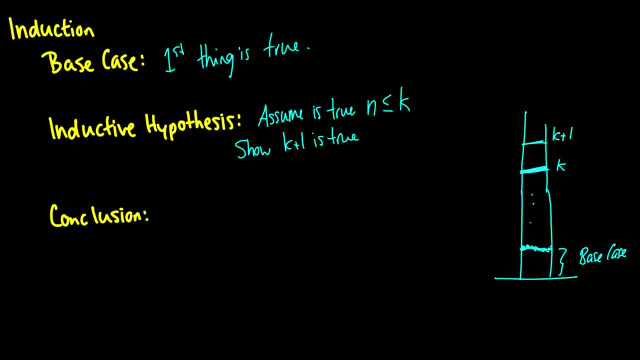 So sort of what this is saying is that okay, if I'm at some random step, then I should be able to get to the next one, And that's all it's saying. It's saying, okay, if I pick an arbitrary step, then I should be able to lift my leg. 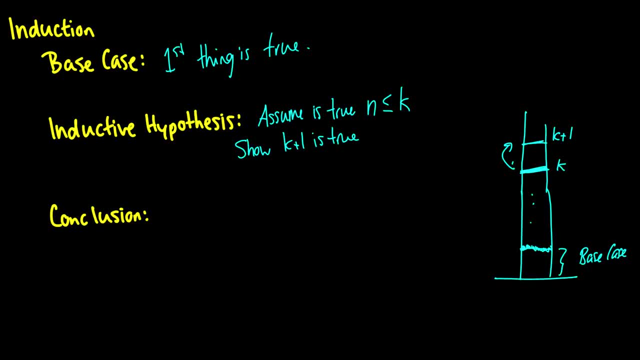 and there should be some next step that I can get to. And if that is true, then you conclude that every n is true, Which means that if the first step is true and from some arbitrary step I can get to the next one. 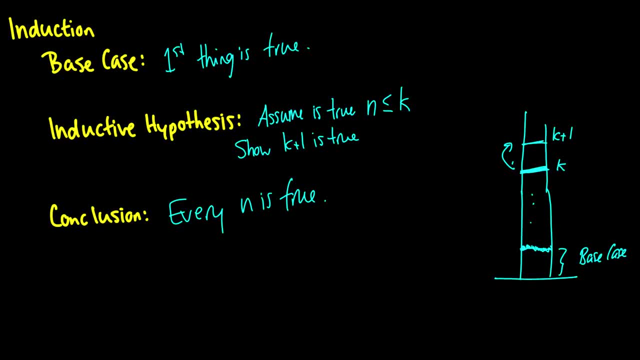 then, clearly, this is a full functioning ladder and I will be able to get to the top of my ladder. Now, why is this the case? So you prove that you can get on the ladder. And then you prove: hey well, since I got on the ladder, if I go to any random step, that I can go to the next one. 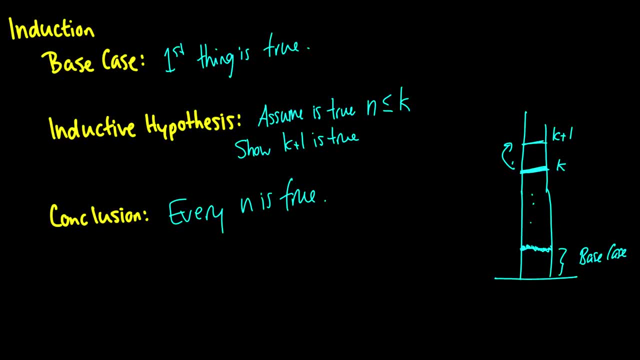 why does this show that? okay, I can go from this first step to the second step. Well, if you're not sure, then we say, okay, well, we'll just say that our k was this first step. Okay, well, then I can get to the next step. That's fine. Okay, now that I'm on the second step. 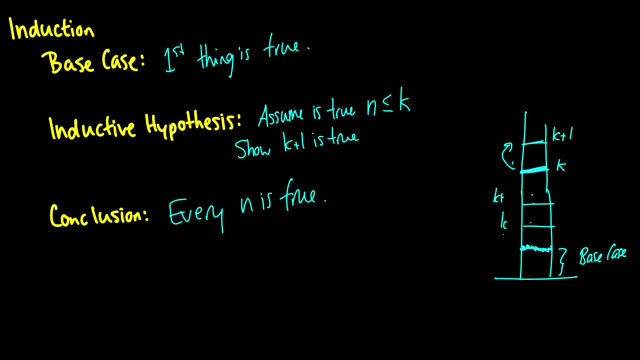 let's make the second step be k, and we know that k plus 1 is true, so we can get to the next step. And this will just keep going on and on and on forever, And eventually you're going to get to. 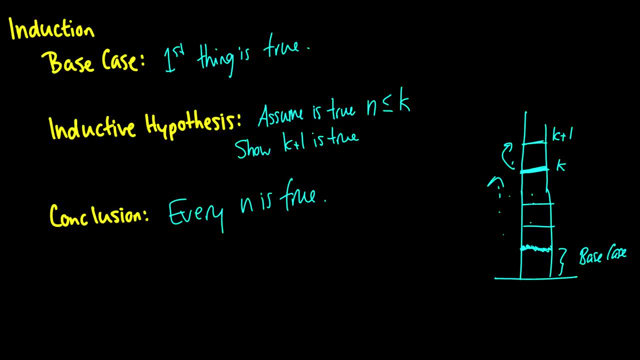 the very top of the ladder. So that is the ladder analogy for induction. And if you want to see a logic example, you can go to the very top of the ladder. And if you want to see a logic example, check out the Natural Deductive Logic series. 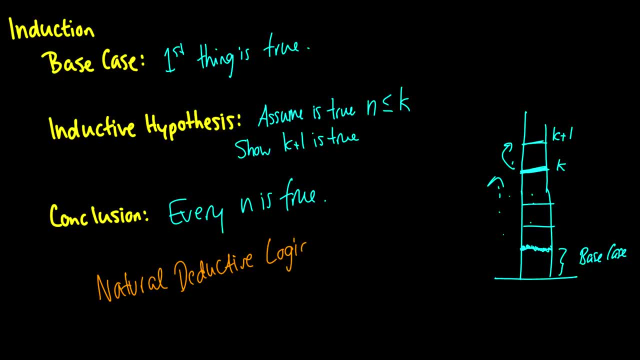 on my channel. It is actually just a video called Mathematical Induction. I literally go over the same example with the ladder, except I do a logic proof instead of what I'm about to show you, and you can get yet another example, since I think a lot of the courses I'll be doing will require. 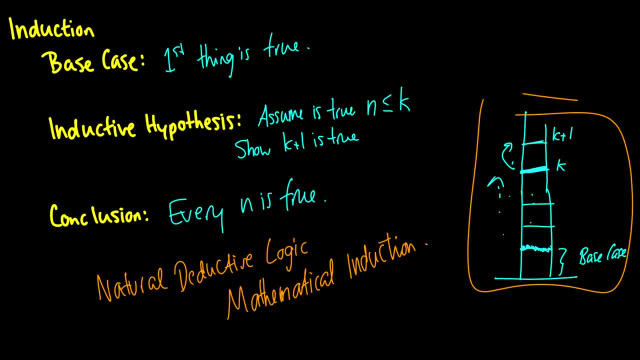 least one video on mathematical induction. so hopefully you'll have a bunch of different examples. And of course you can just check this out very easily at trevtutorcom. I'm just going to plug myself in there. If you go to the logic page, mathematical induction- it's right there So you can check out a. 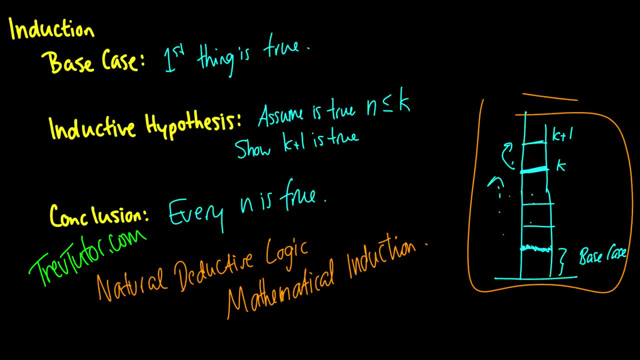 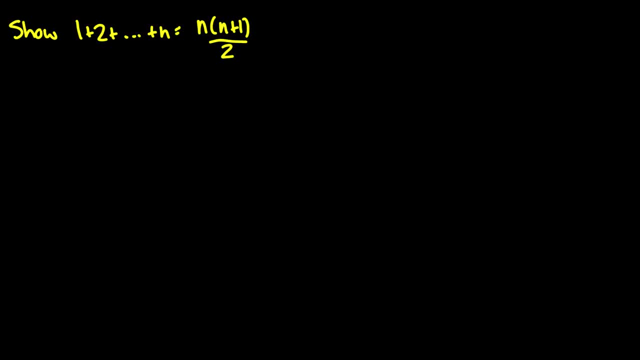 propositional logic example after this first one. Okay, so let's show that 1 plus 2 plus dot, dot, dot, all the way up to n, is equal to n, at times n plus 1 over 2.. Well, we need to start with a base case and we need to assume that n is equal to. 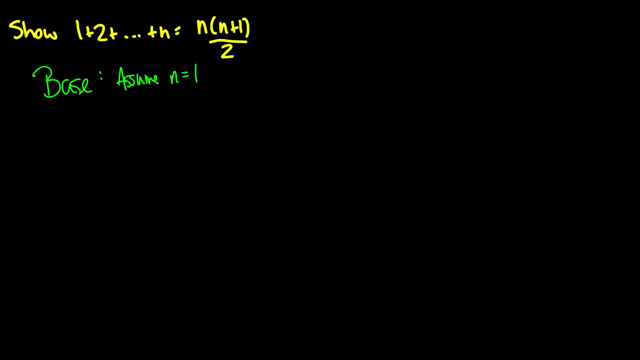 1.. Now we have to prove that this holds for the first number. So what we're saying here is that 1 is equal to 1 times 1 plus 1 over 2.. Well, which is equal to, of course, 1 times 2 over 2, which is just equal to 1.. So this 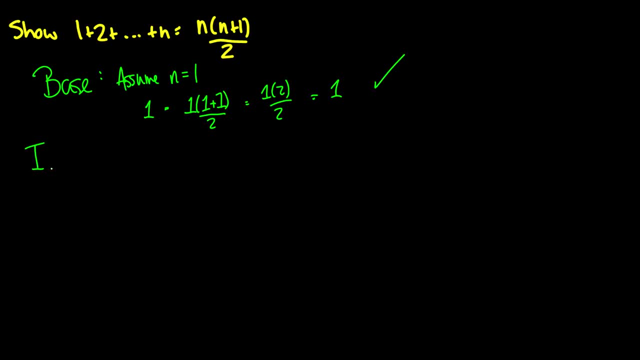 is good. Now the inductive hypothesis is where people get a little bit tripped up the first time. So what I do is I say: assume n less than or equal to k is true. So what this means is that 1 plus 2 plus all the way up to k is equal to. 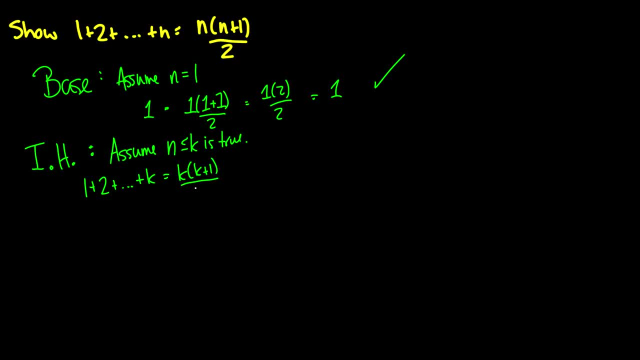 k times k plus 1 over 2.. Okay, so now I have to show that k plus 1 is true. So what does this involve? Now? essentially, we're going to go one step further. So we say that 1 plus 2 plus all the way up to plus k plus k plus 1 is going to equal k plus 1 over 2.. 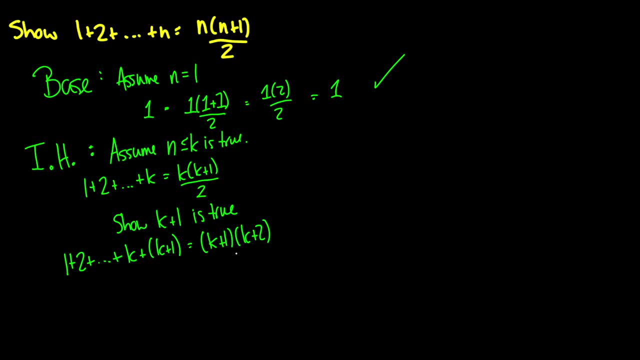 k plus 1 times k plus 2 over 2.. All I did here was I put in k plus 1 per k. That's all I did, Okay, so where do you go from here? Well, the assumption is the most important part of a good 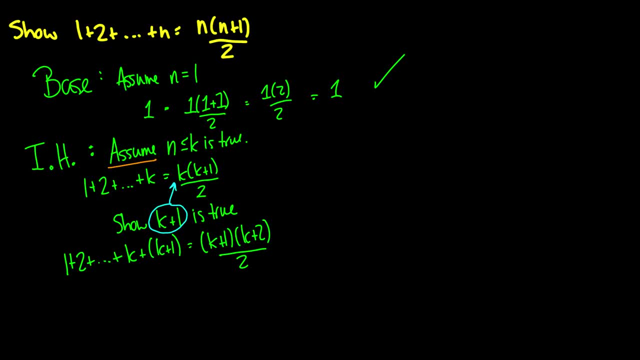 inductive hypothesis, since what we have here is that this part right here, this 1 plus 2 plus 1 plus all the way up to k, is equal to k times k plus 1 plus 2.. This is part of our assumption. So what we can do is we can plug this in So we have k times k. 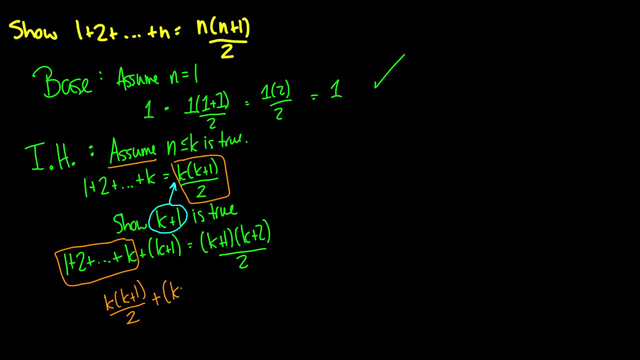 plus 1 plus 2.. We can just add k plus 1 and now we just need to show that this equals k plus 1 times k plus 2 divided by 2.. So we can do some nice algebra here and we will get that k times k plus 1 times k plus 1 divided by 2 is equal to: 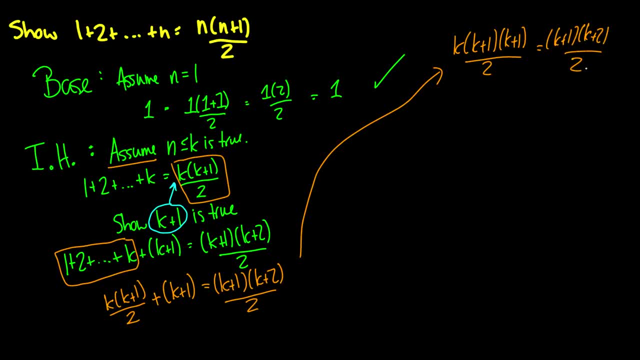 k plus 1 times k plus 2 over 2.. Again, I just found a common factor and put it all to this value. So on the left, here we have: k squared plus k plus k plus 1 over 2 is equal to well, let's, let's factor this out: k squared plus 3, k plus 2 over 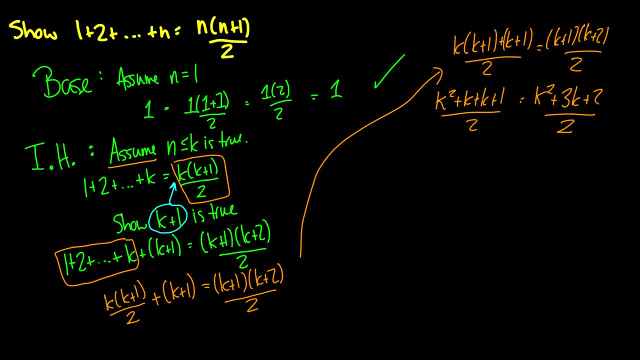 2. And when I take a look here at this, I see that my math is just a little bit wrong. This should be plus 2 times k plus 1, when I fix my mistake, which means this will be k squared plus k plus 2k. 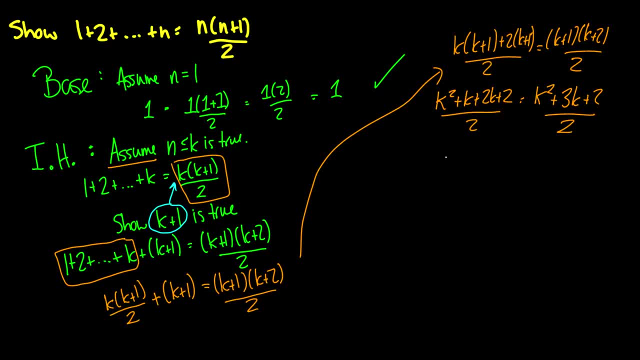 plus 2, and we can see here that if we collect like terms on the left side, they will actually equal to each other, which means that we have shown that k implies k plus 1 to be true, which means that we have shown inductively that this statement is true. 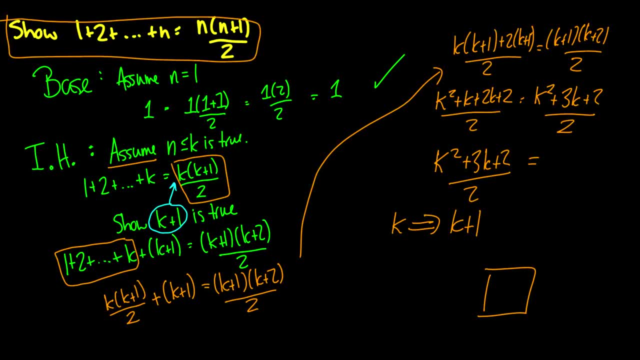 And I know this might seem a little bit confusing to people- like, wait a second, why does this work? Like we've assumed that this is true right here, but then we just use it in the, we use it in our proof and it doesn't seem weird. It seems like we're making a circular. 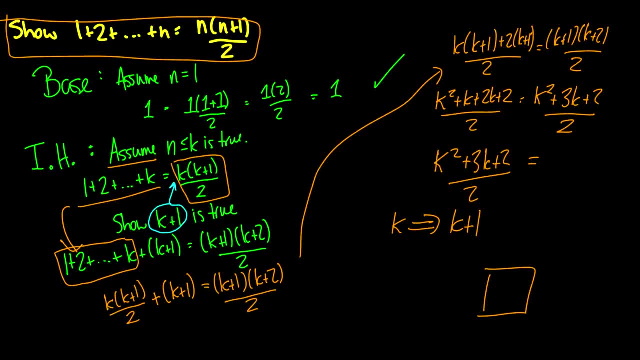 argument, and that is one of the first things that you'll say when you first see the proof. isn't this a circular argument? But again, it's just logic If we say, oh whoops, that is another proof there. If we say that phi arrow, psi is true, then if we assume 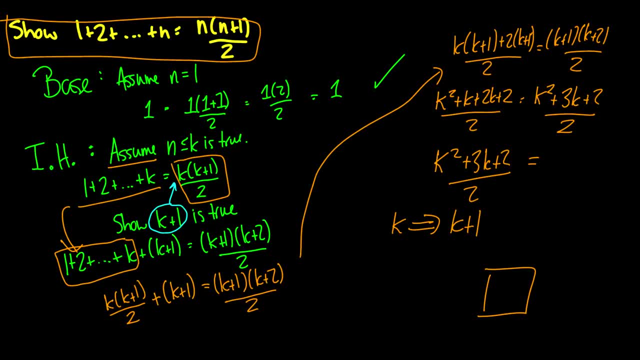 phi, we should get to psi, and it's a hypothetical thing. We've hypothetically assumed the first part is true. therefore, is the next part true? And if that is the case, well, everything was arbitrary, so the whole thing is true. So hopefully you followed that. If not, you can always leave. 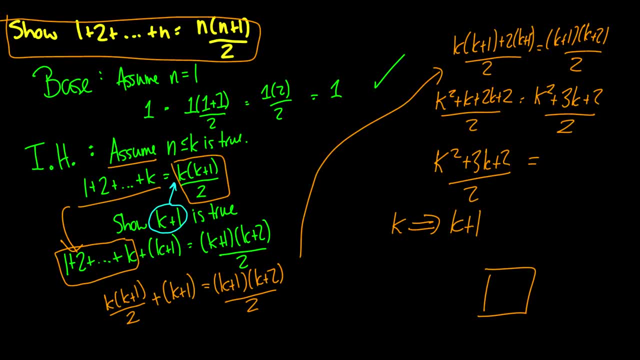 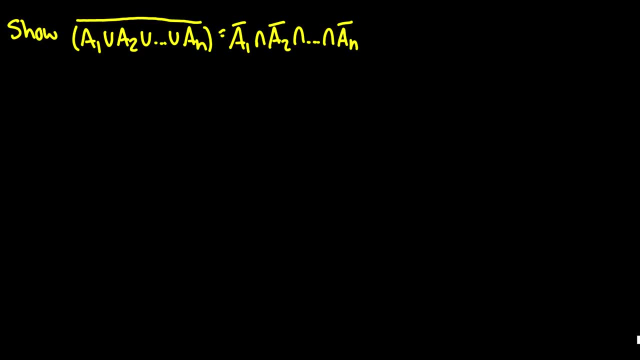 comments. but what I'm going to do is I'm going to do my favorite exam question ever. I love this example. I'm going to do my favorite example. I'm going to do my favorite example. I'm going to do my favorite exam question. I think it's great. Show that the complement of a1 union a2 all the way up. 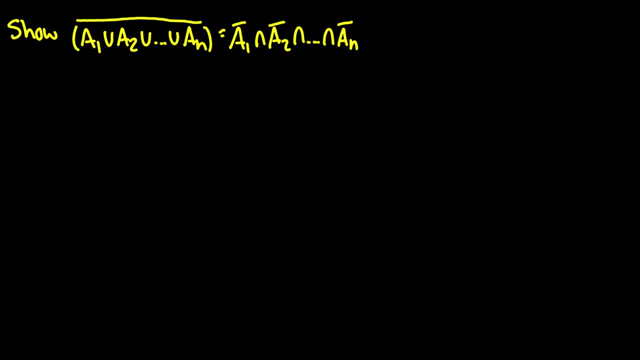 to an is equal to the complement of a1 intersect the complement of a2, intersect dot, dot, dot all the way up to the complement of a sub n. So this is a set theory proof, and the reason I like this is because a lot of people don't see it coming and they're a little bit confused on what to do. 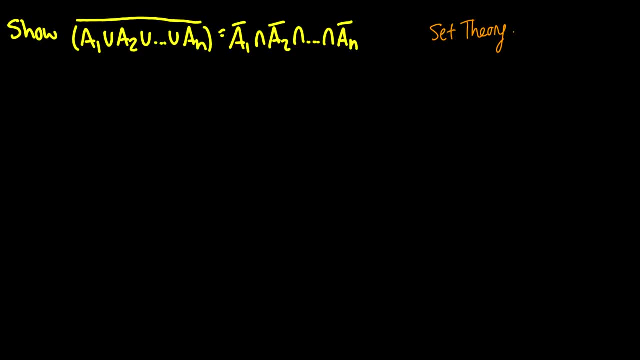 because it's induction, which is weird. Okay, so for the base case, what's interesting here is saying n equals 1 is true is a little bit weird. What we have to do is we have to show that a1 union a2 is equal to the complement of a1. 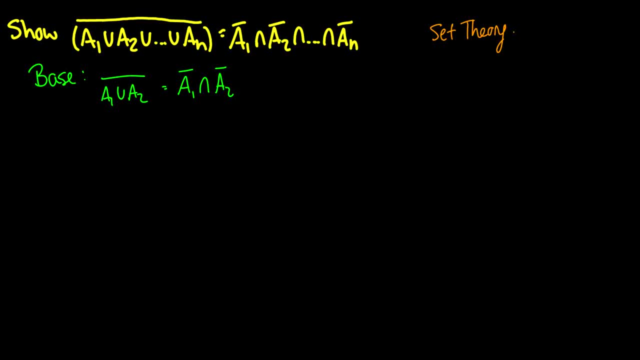 intersect the complement of a2, which we know just by the Morgans that this is true. So the base case is handled. The inductive step is a little bit more interesting for this, because we assume that a1 union all the way up to a sub k, the complement of that is equal to this whole thing right here, which seems like. 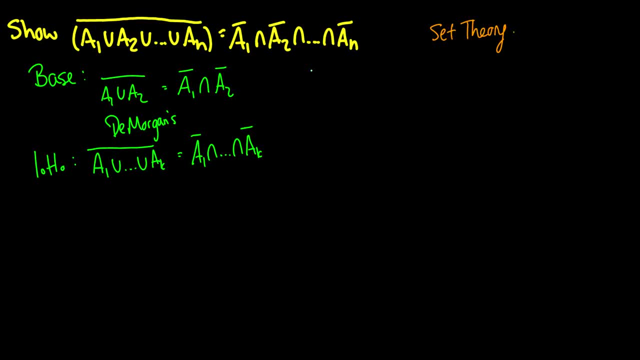 well, I just proved the result, but that's not really the case. And you're saying, well, wait, wait, why do I even have to do this? Well, I just proved the result, but that's not really the case. 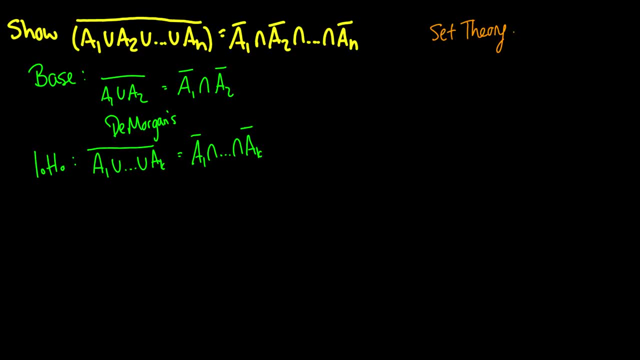 This proof is ridiculous, and I will admit it's a tiny bit ridiculous, but follow along here. So we just assume this first part is true. Now we have to show that it's true if we add one more in. So what we do is we say, okay, let's do what we did before and get this whole complement. 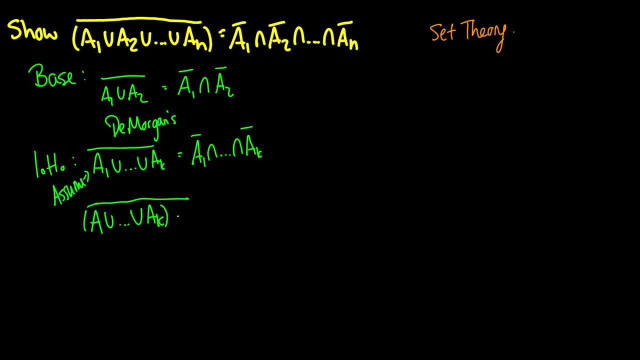 but let's bracket the first part, and then we'll put in this union for ak plus 1, and then we'll put in this union for ak plus 1.. Okay, well, let's just do DeMorgan's here, just like we did in the first part. 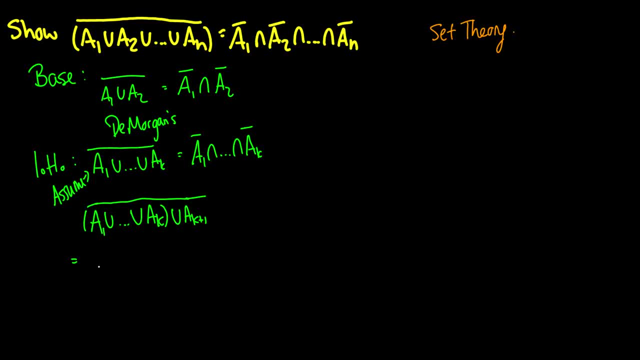 Okay, so with DeMorgan's we have this whole first part. We're not going to do anything with the union yet because we can't, We can't do it yet. But then this second part becomes okay, an intersection with ak plus 1 and the complement of that. 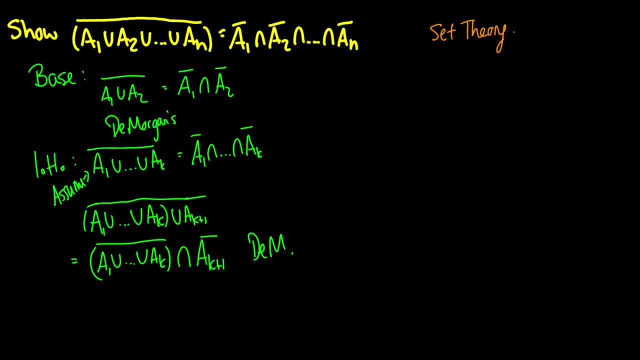 Well, that's fine and that's by DeMorgan's, But we know with our assumption here that this other section is going to hold as well. Therefore, this complement of a1 union all the way up to a sub k is actually just going to be the complement of a1 intersect.